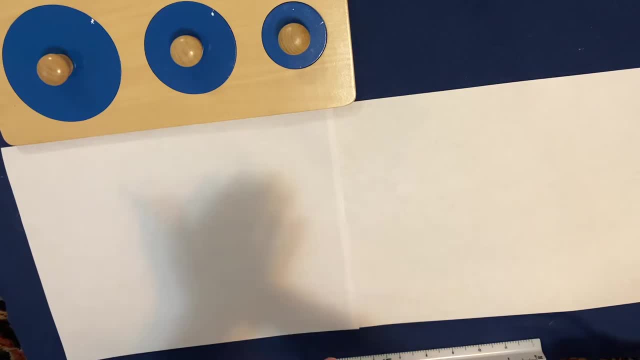 Area, radius, diameter, circumference and center. Okay, you need to know what all five of those are. If you're not sure, that's okay, Just go back to the parts of the circle, practice that lesson a little bit more and come back and join us. 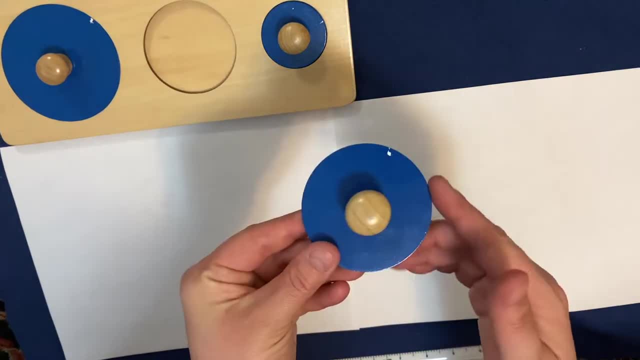 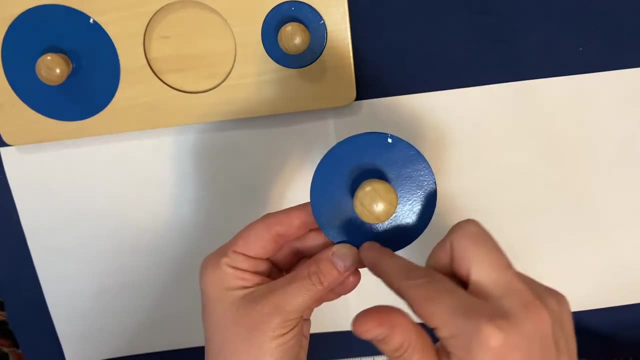 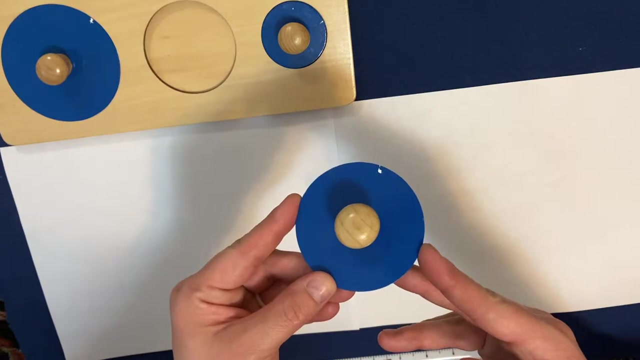 So, if you remember, the circumference is the line all the way around the circle And today we want to learn how to measure that line around the circle. Now, when we have a rectangle or a square or a triangle or trapezoid, octagon, nonagon, we can measure. 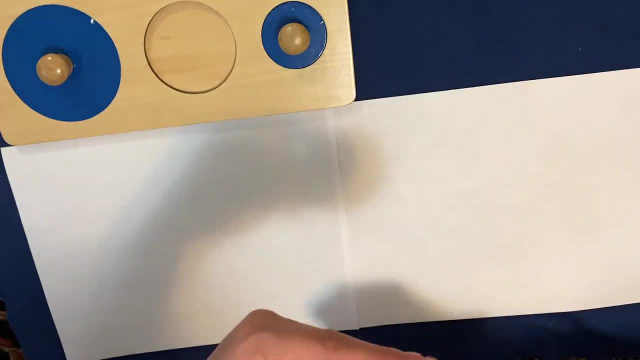 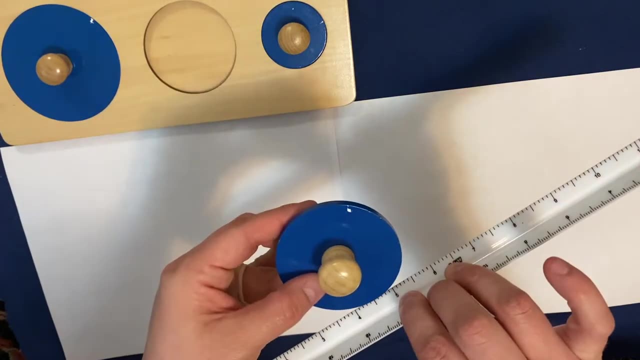 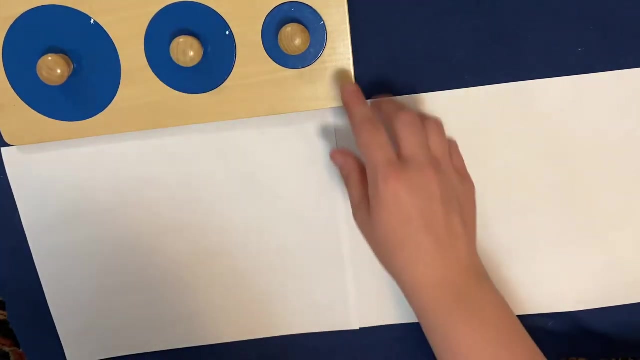 the perimeter just by using a ruler and marking down how many inches or centimeters it is all the way around With a circle. we can't use a circle with a ruler because it's rounded, So I'm going to show you what we can do today. So I have three circles here. I've marked them. 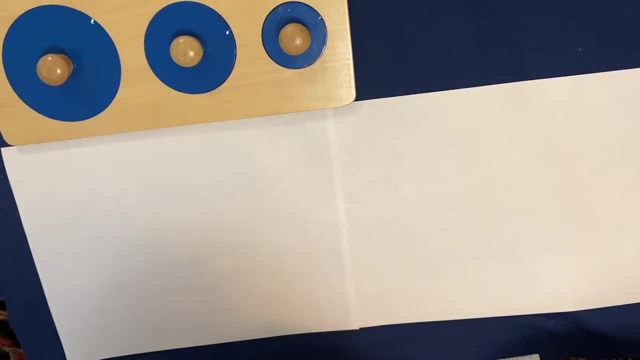 each with a little bit of chalk, because it'll rub right off. You don't want to mark the circles with anything permanent, You want to mark them with a little bit of chalk, because it'll rub right off. And it especially fits something like this: This is Emily's concentric circle puzzle, So I want to 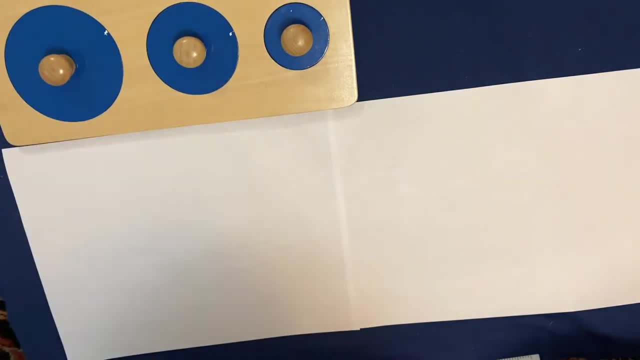 make sure that I can return it to her with no marks, mark-free. So the first thing we need to do is I've taped two pieces of paper together in case I get circumferences that are kind of big, And I am going to draw a straight line. Doesn't matter how long it is. 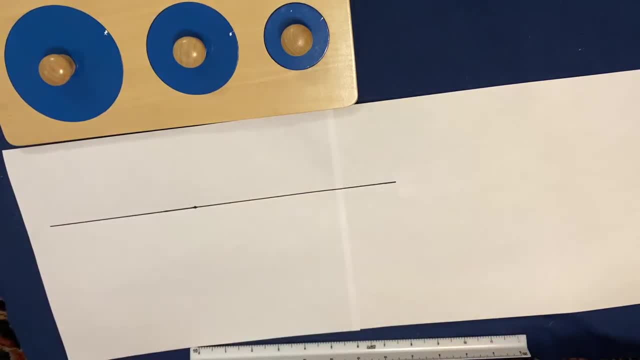 just a straight line like that, And I'm going to put a dot at the very end. Okay, Now I'm going to take my middle circle and I'm going to place this white mark right on the dot, And I am going to very carefully. 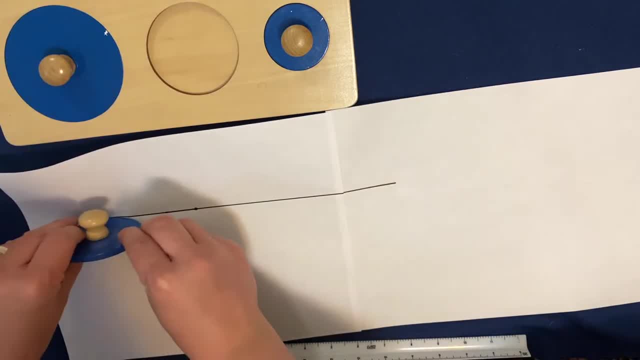 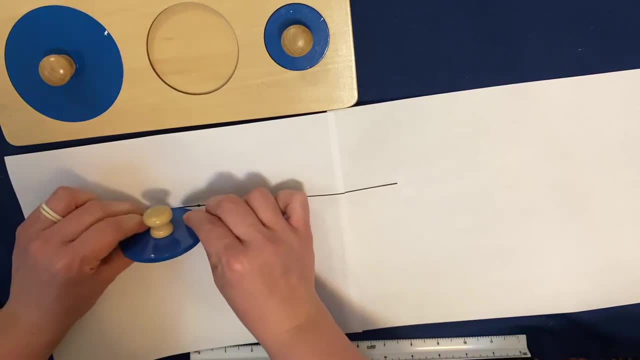 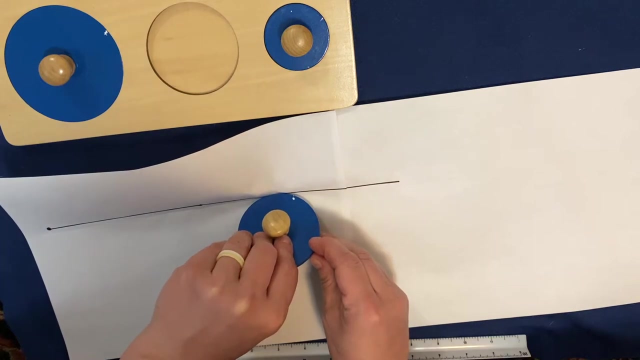 roll my circle without letting it slip or slide, which can be pretty easy to have happen. Okay, So I'm about halfway. See my white point. I'm going to keep rolling and stop. Can you see the white point on the line there? 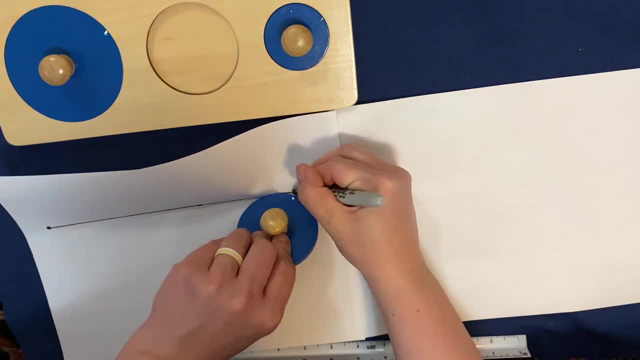 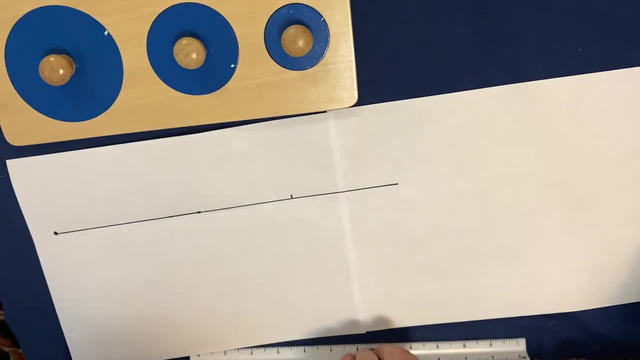 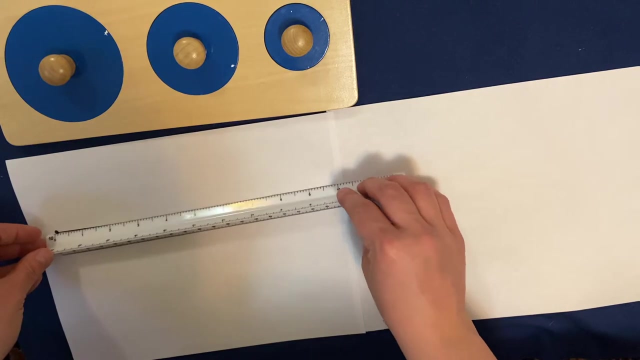 I'm going to take my marker and I'm going to mark where that white spot landed. Okay, So I'm going to take my ruler- I'm going to use inches today because I can't find my good centimeters ruler, Ruler, sorry. And I can see that. 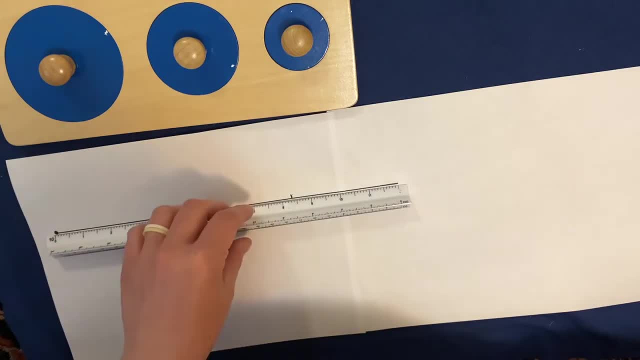 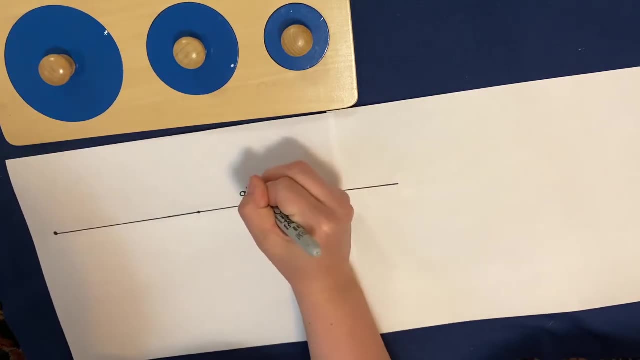 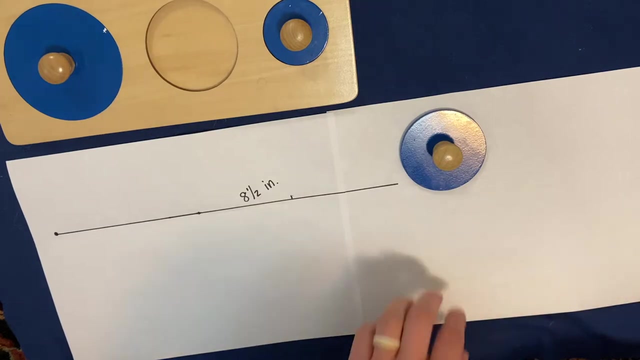 it's about I don't know. It's pretty close to eight and a half inches, So I'm going to write eight and a half inches. All right, I'm going to use this red card. Want to say green and white doesn't fit. 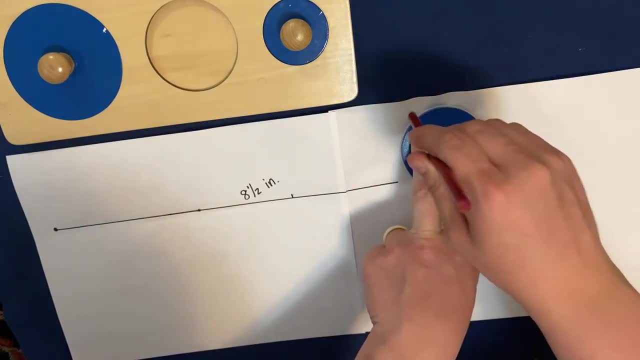 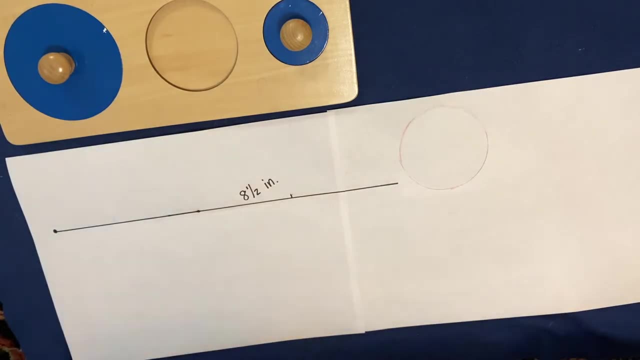 I'm going to carefully trace my circle. Okay, So my circle, let me see It's a little bit smaller. My square would have a chain mark on it. I'm going to just let it slip. see that it's kind of light. we know that my circle, the circumference which I'm 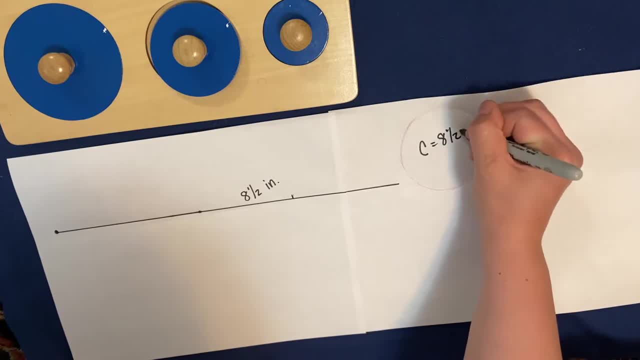 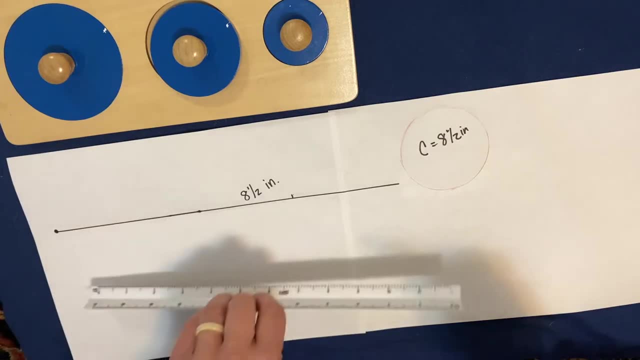 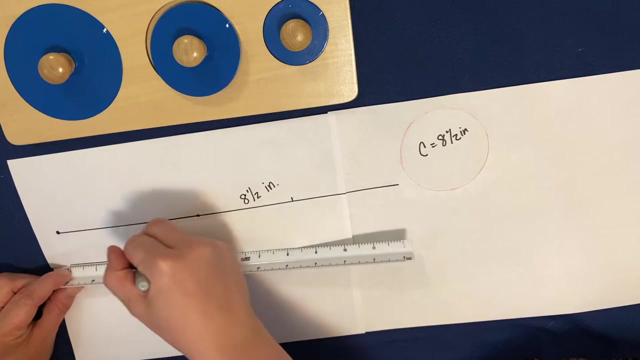 gonna say: is C equal to eight and a half inches? okay, so let's go ahead and do another one. I'm gonna draw another straight line. I'm gonna do my little baby circle. this time I think my line it's a little hard. I'm on the floor in a 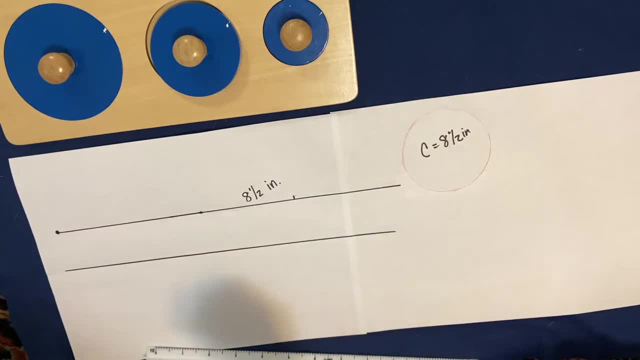 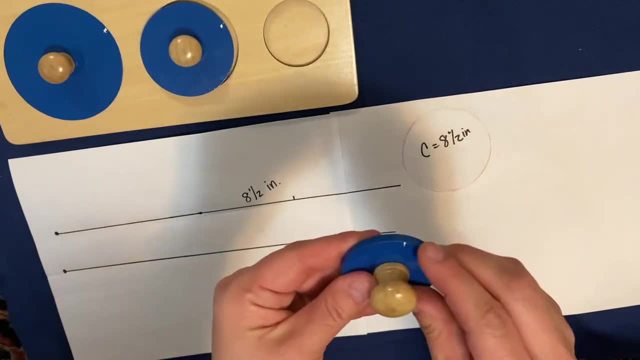 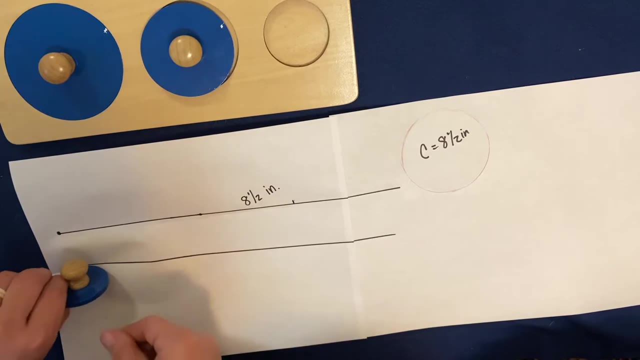 rug and gets kind of bendy and I'm gonna put a dot down here. I am going to take my baby circle, my white spot, I'm gonna put the white spot on the dot and I'm gonna start to carefully, carefully roll. it's really easy for it to slip and 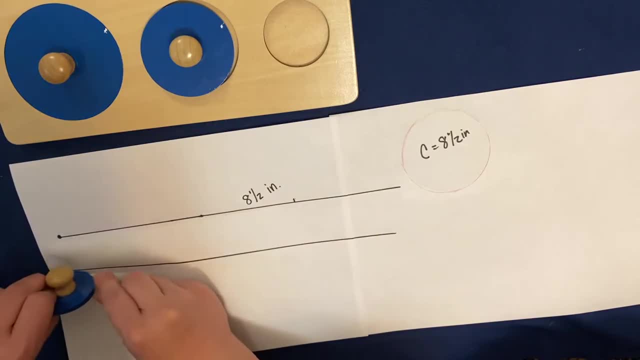 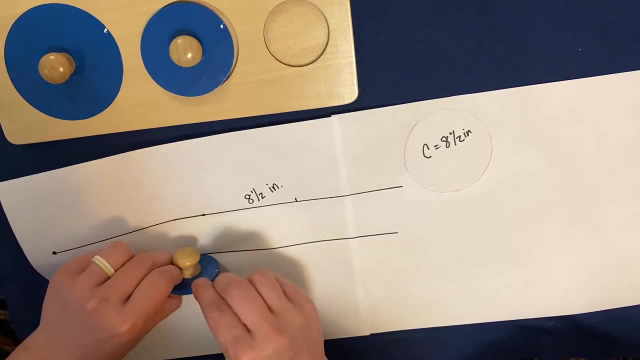 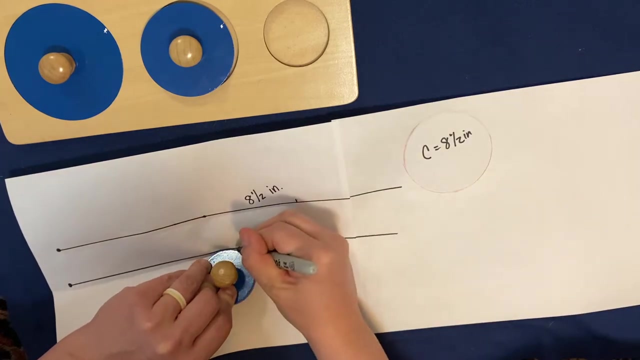 slide like that. so it can take some practice, but I find that pushing down on the paper helps me not slip and slide, because slipping and sliding is going to have you end up with the wrong measurement. so there white spot is on the line. there we go and let me trace. 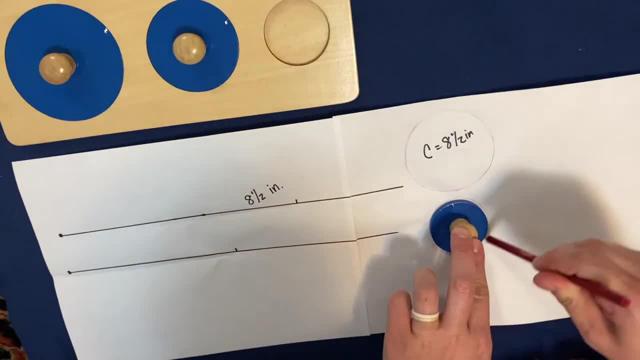 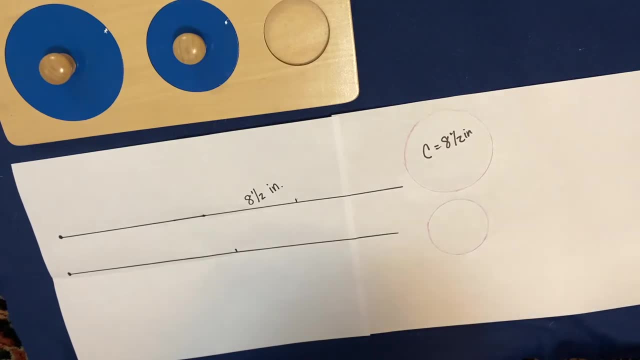 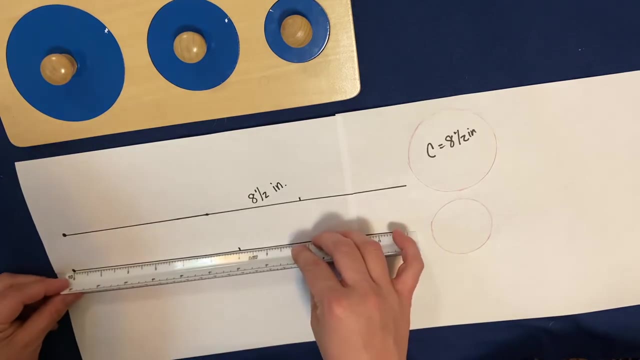 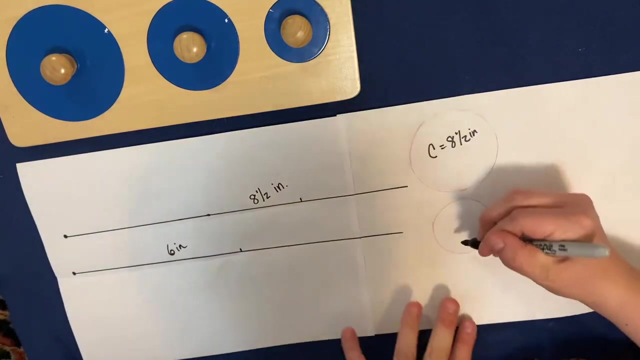 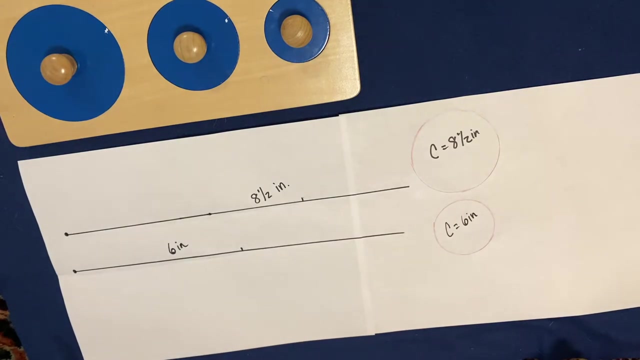 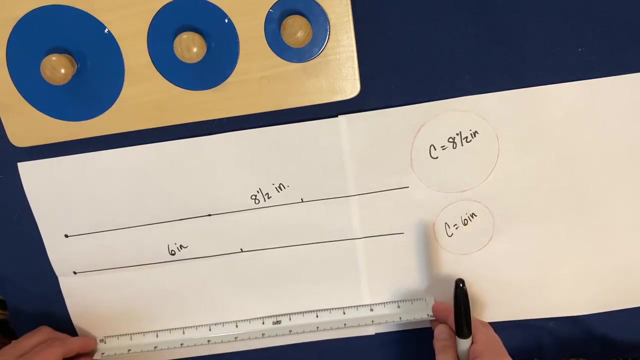 this real quick before I measure it. there we go, and let's go ahead and measure it in our inches, okay, oh, look at that, it's right on six. so six inches, the circumference equaled six inches. very cool, now let's do our our big one. I'm gonna kind of make my line a. 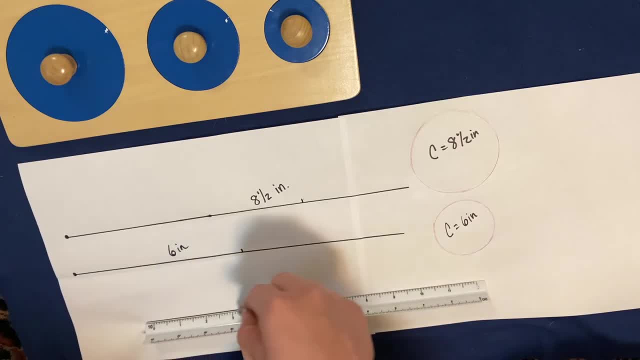 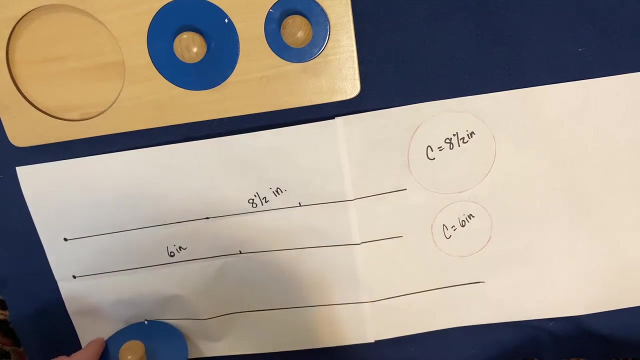 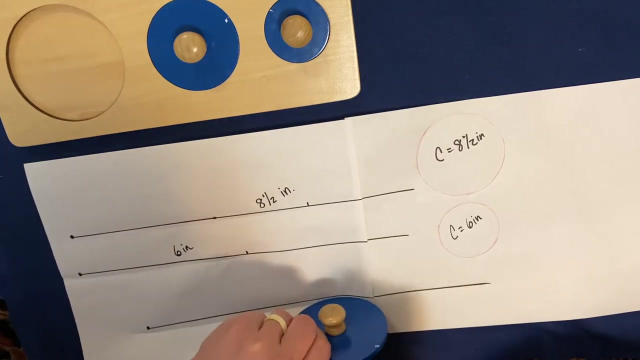 little off-center here. there we go. let's hope that's long enough. gonna make my dot. I'm gonna take my big circle, I'm gonna put the white dot or the white mark on the dot and I'm gonna begin to roll my circle. I think we're just barely gonna make it. yes, see. 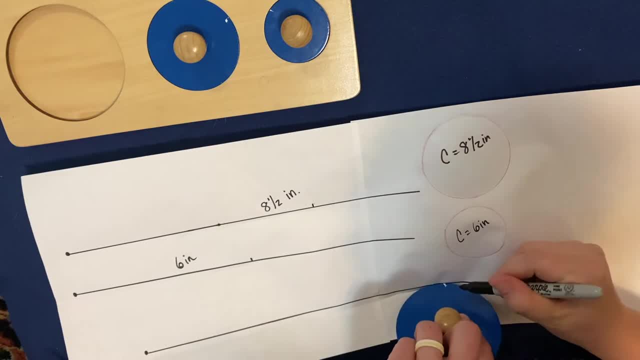 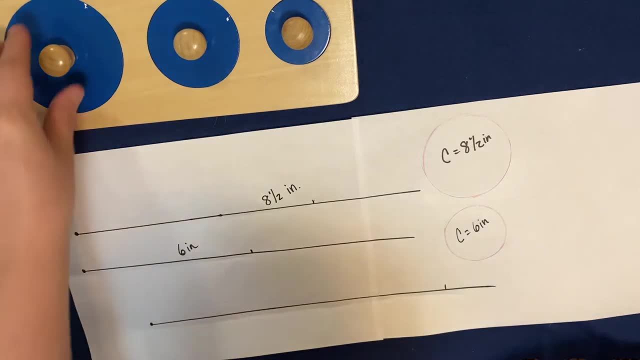 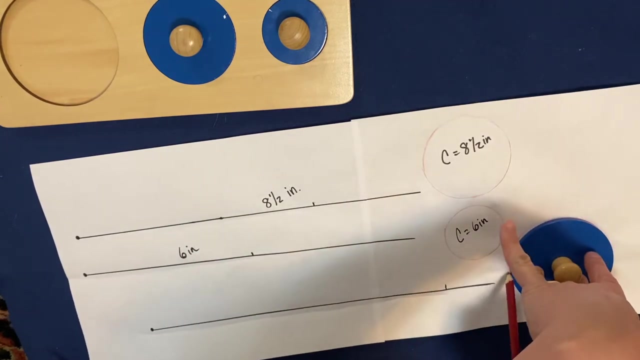 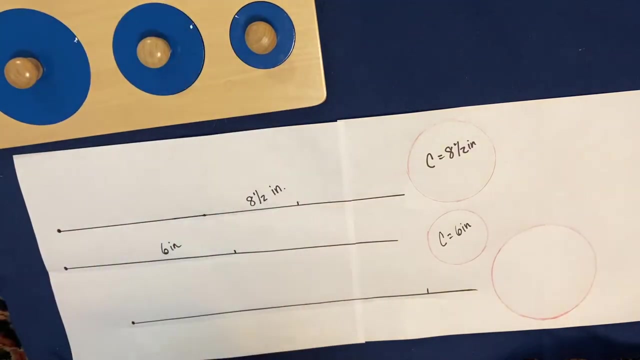 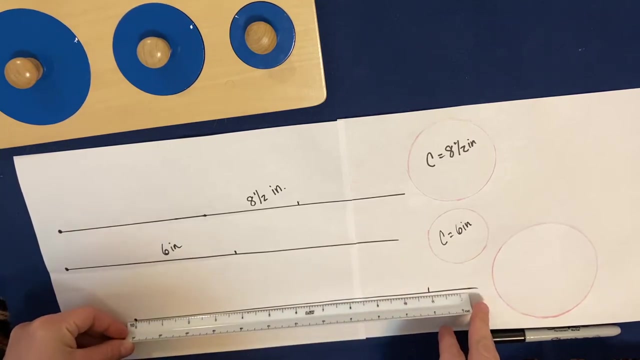 where the white spot landed. I'm gonna go ahead and mark that. there we go. and again, I'm gonna trace it before I measure. there we go. done with our circles, okay. so let's go ahead and measure this bad boy, and that is pretty darn close to 11 inches. 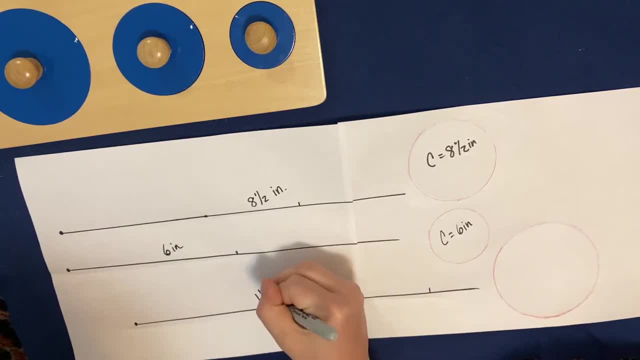 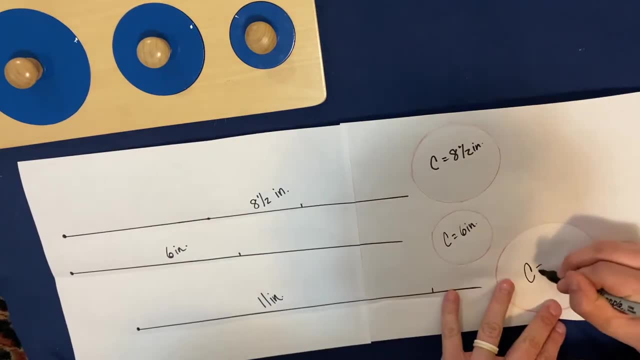 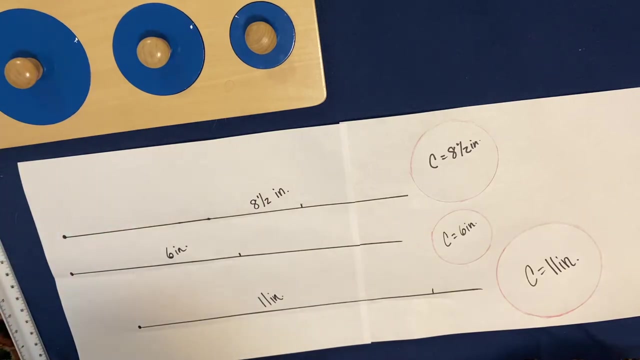 okay, so let's go ahead and measure this bad boy, and that is pretty darn close to 11 inches. 11 inches, alright, 11 inches. so the circumference of this circle equals 11 inches. all right, cool, so you can do this with any circle or cylinder in your house that you would like to do it with. you know, um, you might. 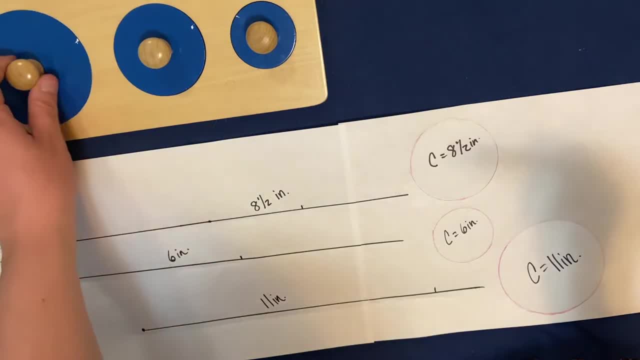 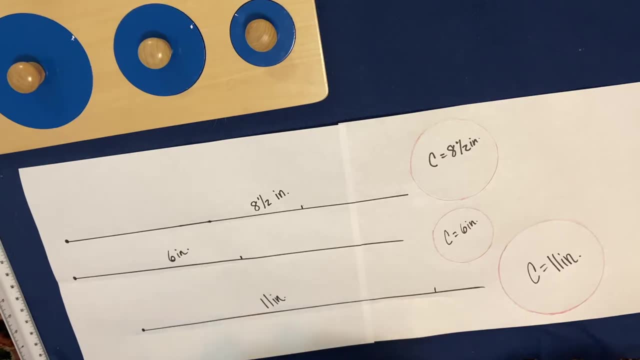 need to tape paper together if it's to be any bigger than this. also, please ask permission if it's going to be in any way big, before you start rolling it out and all that kind of stuff in your house. if it's breakable, if it's. 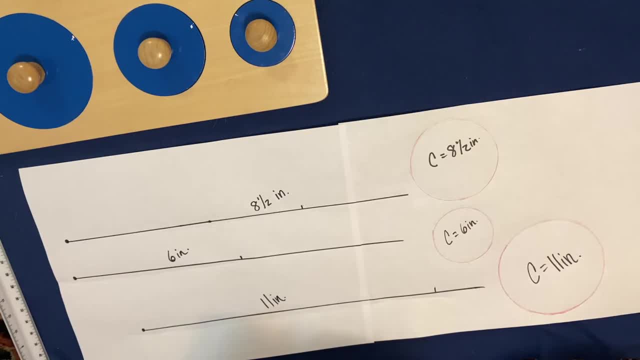 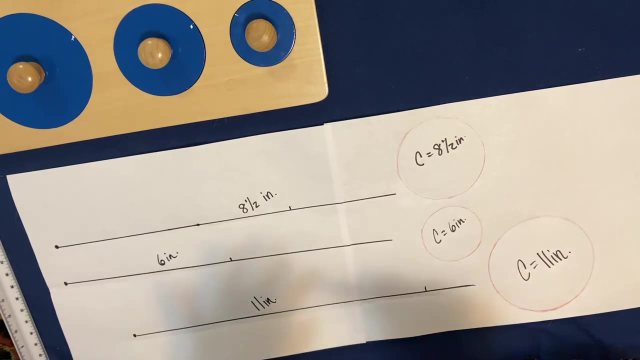 something your parents might not want you to be rolling around. please make sure you ask them first, but you can go ahead and collect as much as you want, and you know this is just two pieces of paper taped together, but you might need three, I don't know. it depends on what you find. so this is the 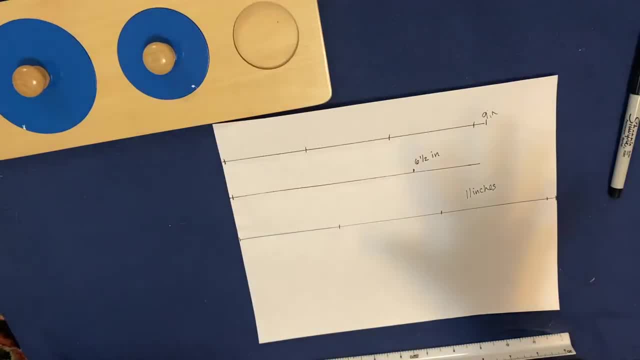 first step. but I want to go ahead and show you one other thing. so I went ahead and redid my lines and rolling and measuring on a hard surface just to make sure that pushing into this soft floor wasn't having an effect. and it turned out that it actually was. I was about a half inch off on both. 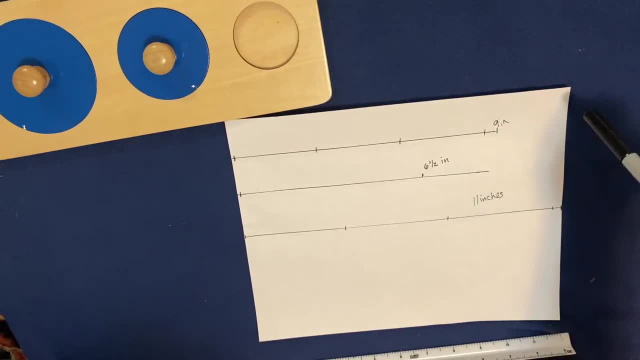 these circles. this one ended up being pretty much right. but so with the medium and small, I was a little bit off and you really want it to be correct, especially when you're doing a lot of work, and you want it to be a little bit off and you really want it to be. 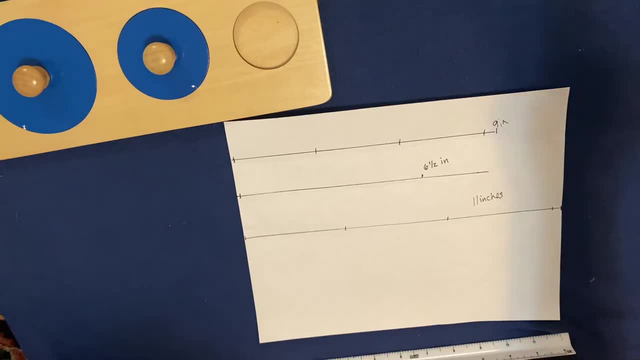 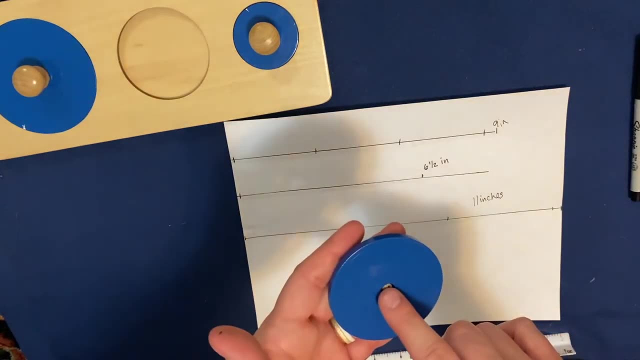 correct, especially when you're doing a lot of work and you want it to be a little bit off, and you. I show you this next part, so I'm happy I went ahead and double checked. double checking it's always a good thing. so let's look first at our medium circle. so do you remember? here is the. 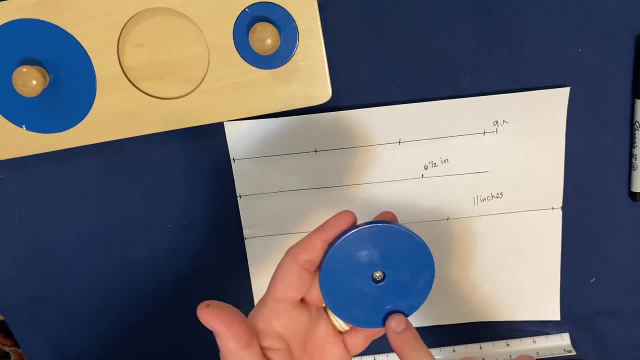 center of the circle and a diameter is a line that goes through the center of the circle and touches two places on the circumference, so it effectively just cuts it right in half like that. so I want to see how many diameters are going to fit inside the length of the circumference. 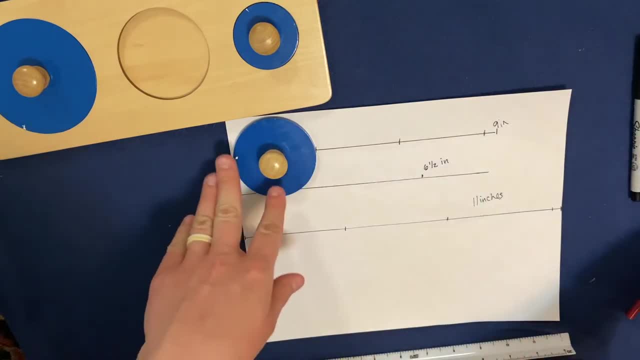 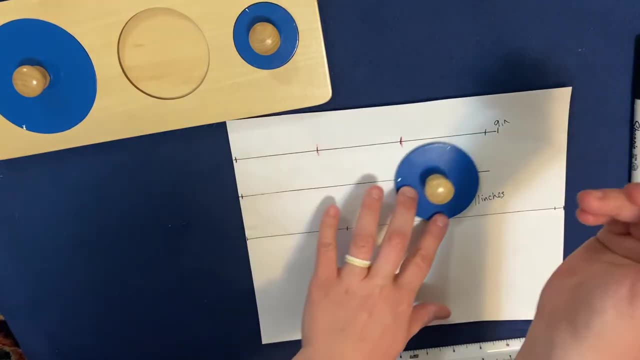 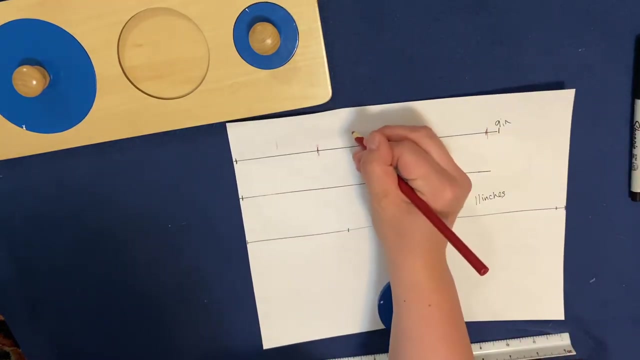 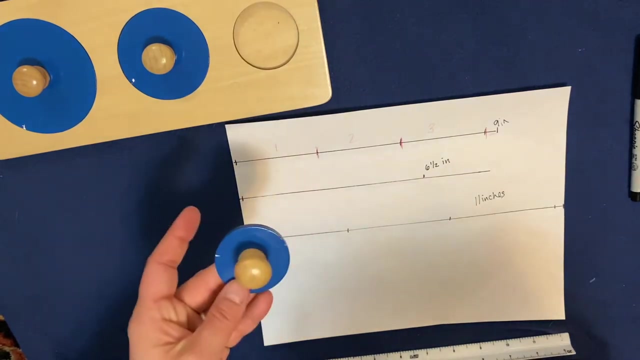 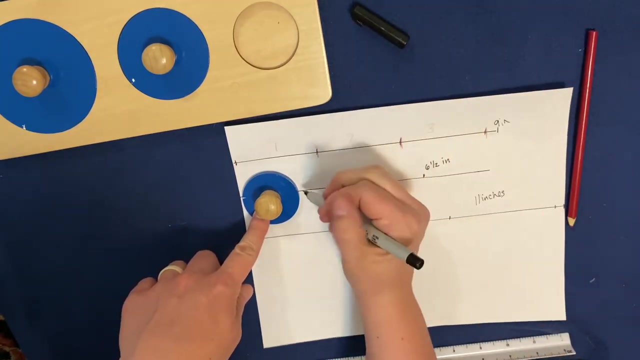 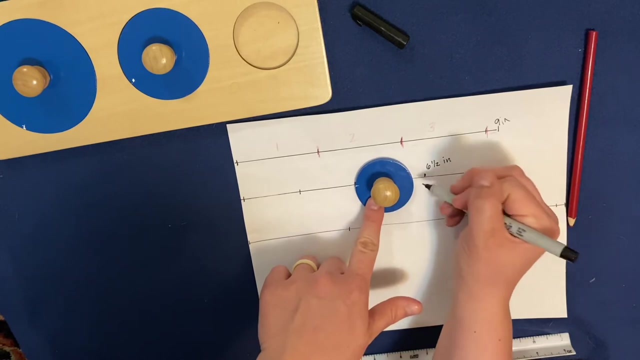 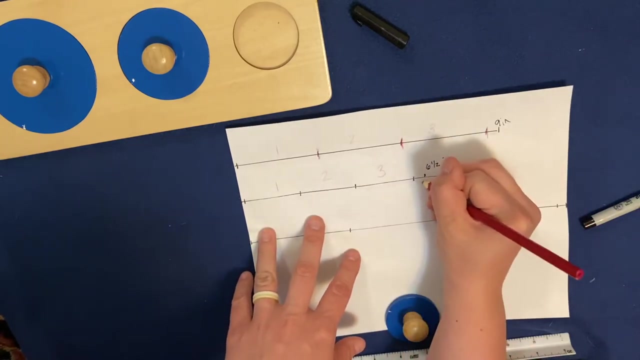 so here we go, we have one, two, three and then there's this little bit left. so one, two, three and then a little bit left over. let's see if it happens again with the small circle and do the darker picture color. first one, two, three. oh, look at that. one, two, three and then a little bit.